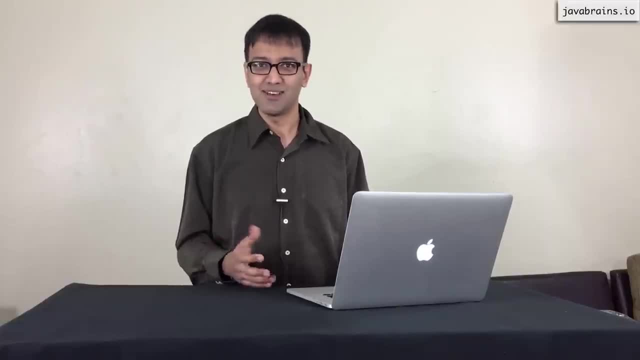 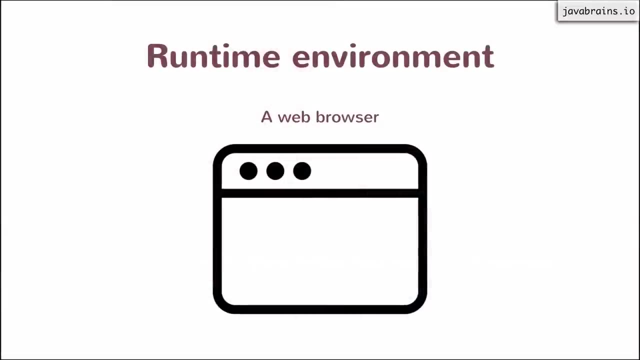 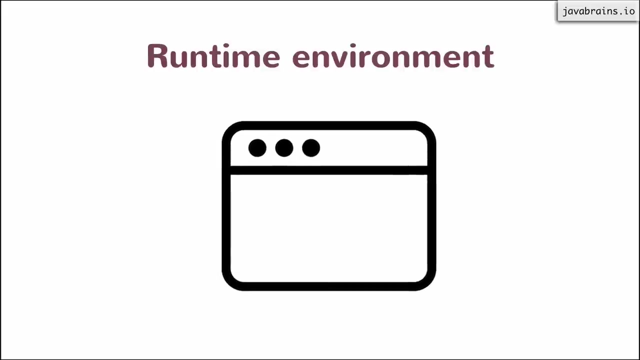 that run complex pieces of functionality on the client's browser, and all of that is courtesy of JavaScript. So how does this work? How is this runtime environment used in a web application? So what usually happens is when you have a web browser and you're making a call to a website, right? 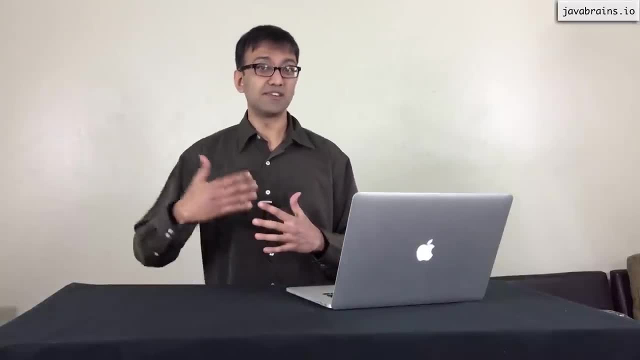 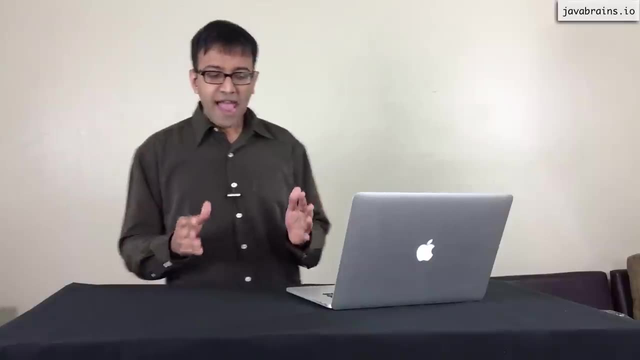 So you type in a URL on the web browser. what happens is the browser makes a request to the server and say: hey, server, give me this page Now. the server responds with some HTML content- HTML as we get from the server as it travels over HTTP. 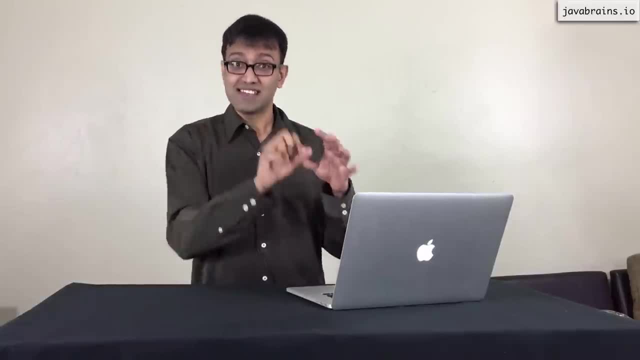 is basically a bunch of text. right, It's a piece of string. that is, yes, less than HTML, greater than So. there are a bunch of tags in it, but essentially it is a string, It's a piece of text. 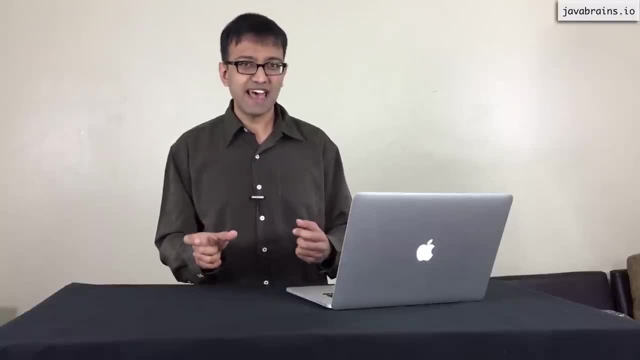 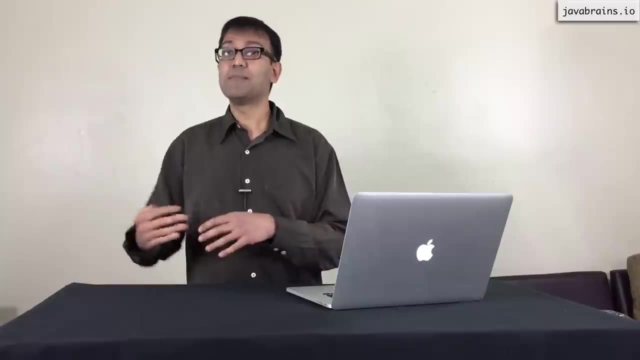 Now what the browser does is it looks at that text and examines those tags. right, If there's an HTML tag and a body tag, a div tag, a paragraph tag, So it takes all those tags and converts them into objects. Each tag becomes an object. 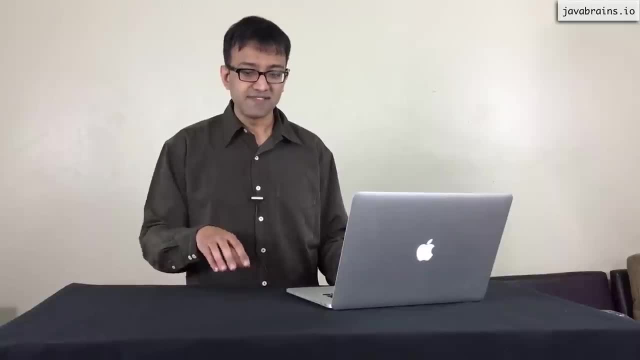 And let's say you have a div and a paragraph inside the div. So the div becomes one object and a paragraph becomes a child object, right? So it basically constructs a tree of objects. This tree of objects is what's referred to as the DOM tree. 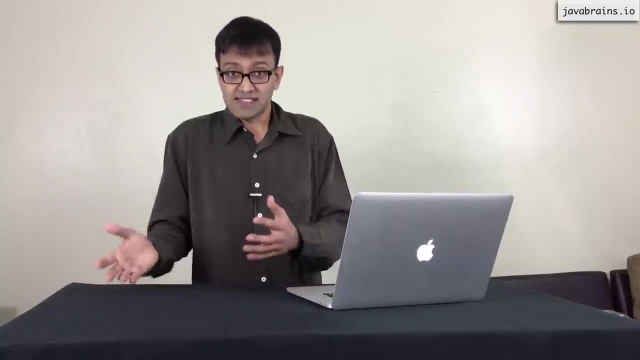 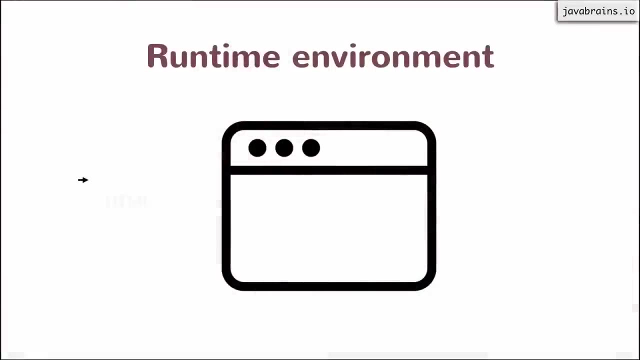 a Document Object Model tree. Okay, it's taking the HTML document and creating an object model out of it. hence the name Document Object Model And that's the tree. So the browser gets HTML. The browser interprets the HTML and builds a tree. 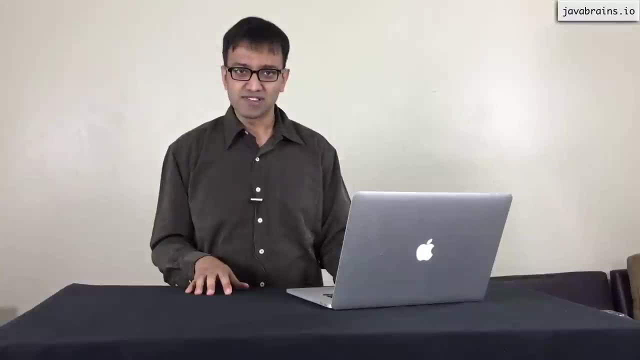 Now, HTML is essentially a static language. If you have just HTML and you have the browser loaded, you get a particular DOM tree right And the browser builds the tree and then renders the view based on it right. So the view is tied to this DOM tree, this object tree. 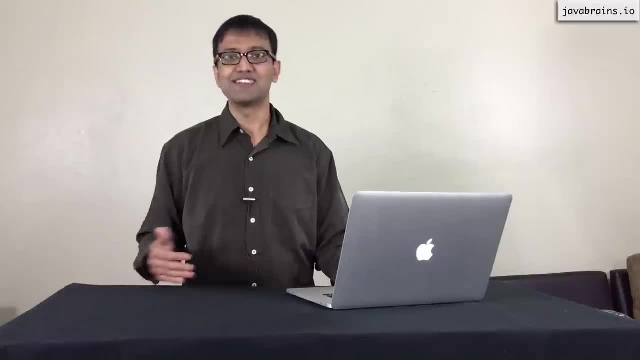 Now, if you load that HTML again, you get the same DOM tree and you get the same view. You load the HTML a third time, you get the same DOM tree and the same view, right? So the HTML is essentially static.